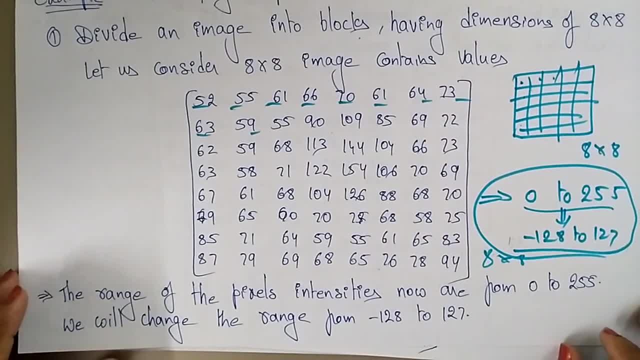 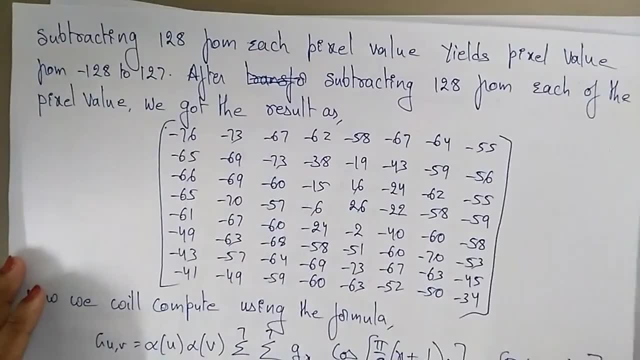 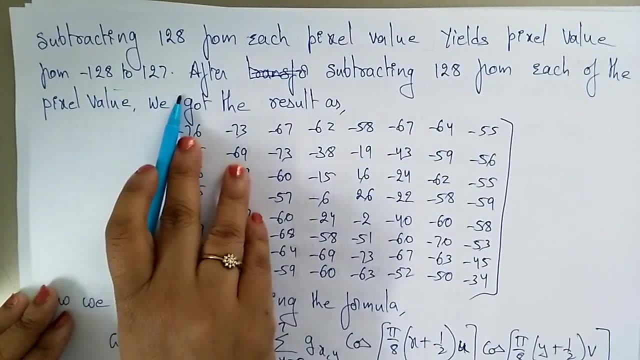 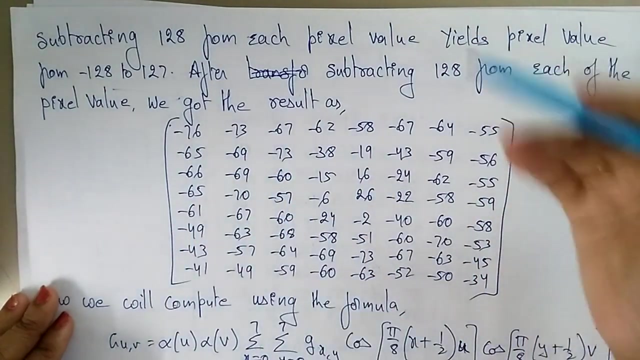 These range into minus 128 to 127. How I can do So? just minus 128. Subtracting 128 from each pixel- Whatever the pixel, that is there that each pixel values- yields a pixel value of minus 128 to 127. So after subtracting, you will got these values. So this is after subtracting. Means I compress the string. I am. reduce that size Means the size has to be decreased. 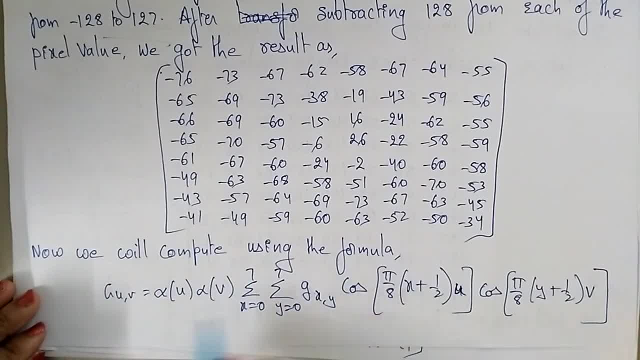 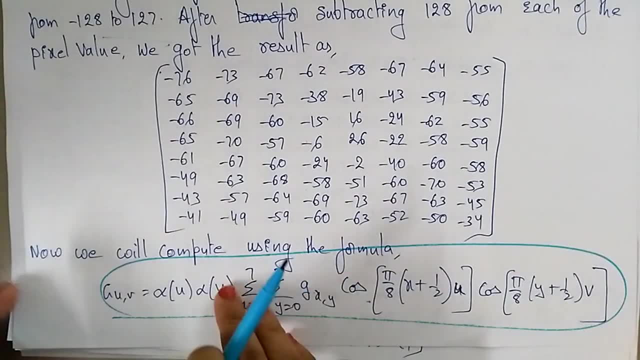 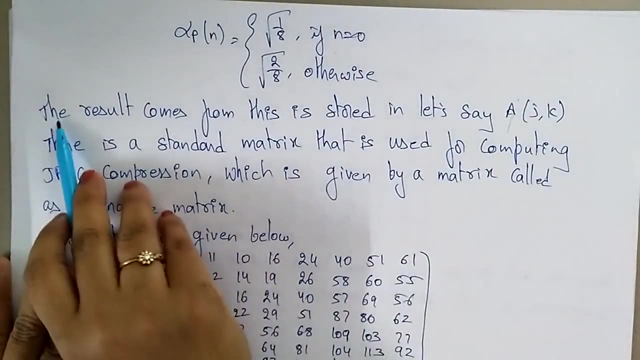 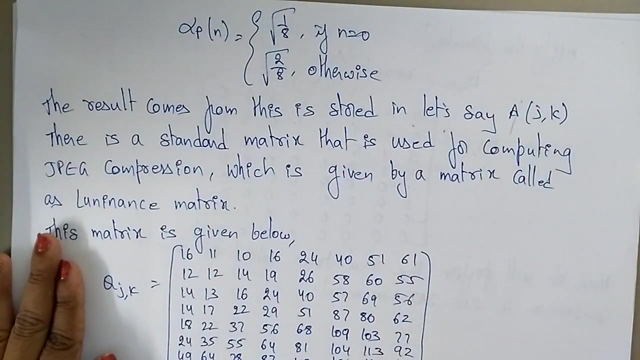 So now apply the formula. Now we will compute using the formula. So this is a formula, because this is a cosine. This is a formula for the two matrices, So apply the formula on that. So this is a formula. Just see that formula The result comes from. this is stored in. Let us take whatever the result, If you apply the formula on that, the new matrix Let us take this is a j comma i. 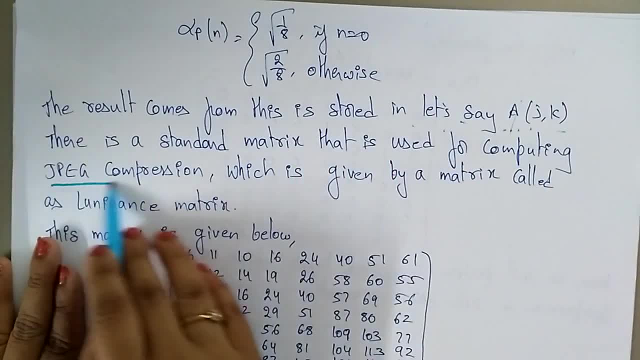 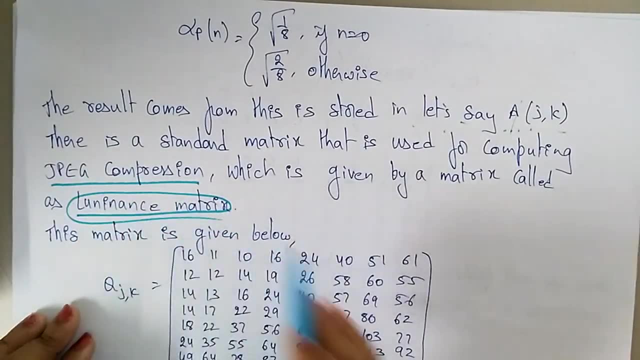 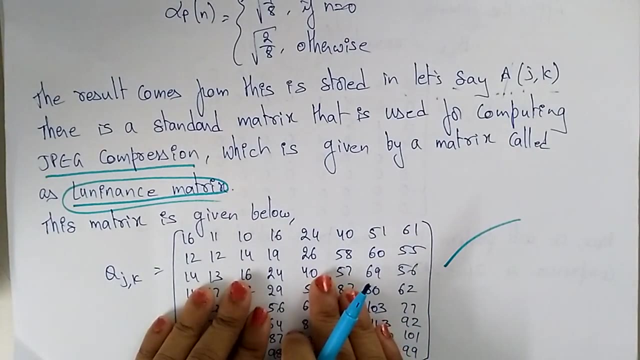 So there is a standard matrix. This is used for the computing JPEG compression. So for every JPEG compression there is some standard matrix, That matrix you call it as a Luninense matrix. So this is this Luninense matrix, This is a standard matrix. Okay, So now take this standard matrix. 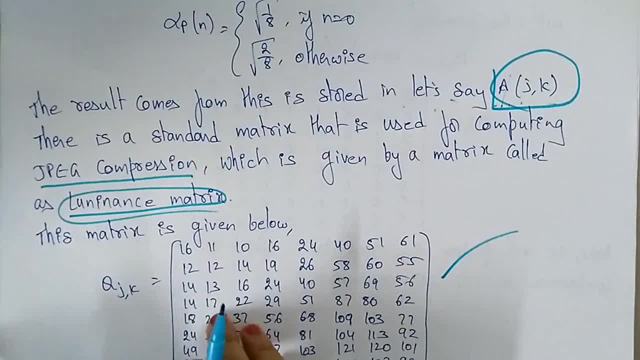 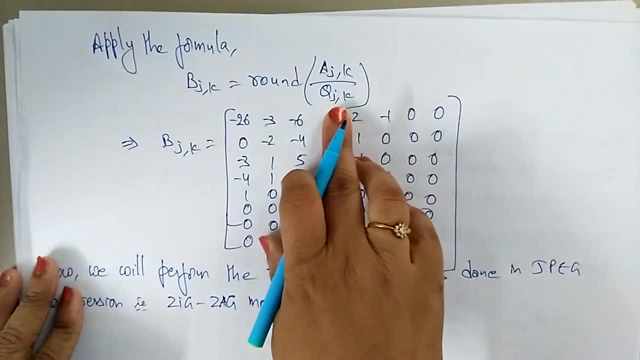 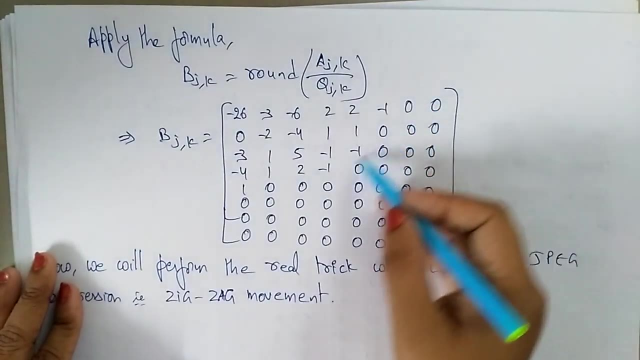 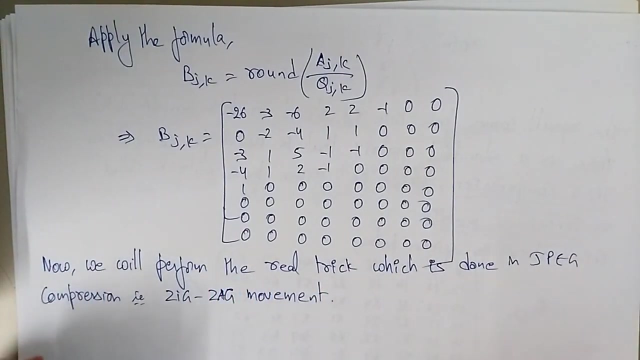 and whatever the new matrix that we came now, apply this formula: BIK round of AJK by QJK. Okay, AJK by QJK. So you will get this new matrix. So did you observe? here You will get all the round. here it is zeros, Okay. So now we will perform the real trick, which is done in JPEG. 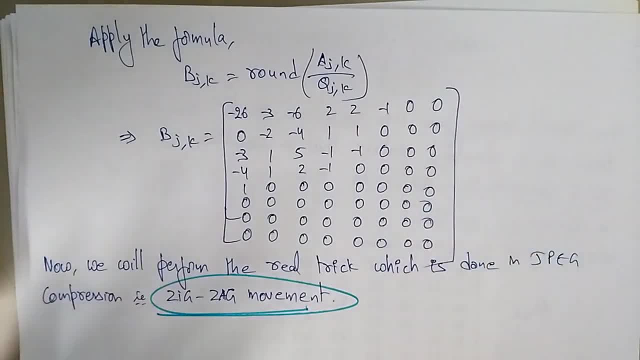 compression. That is a zigzag moment. So, after performing the DCT, this is everything is a DCT technology. So, after performing the DCT, it is a cosine formula. Now apply the zigzag. So how you are going to apply the zigzag, Okay, 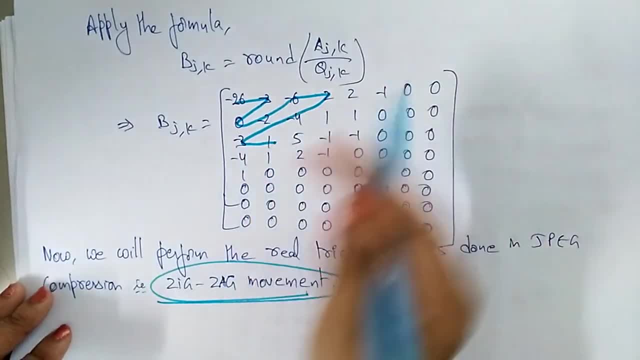 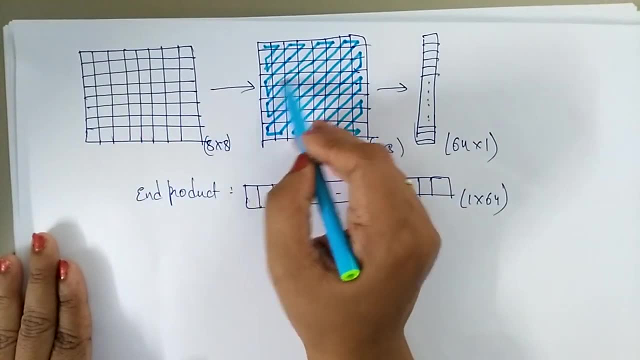 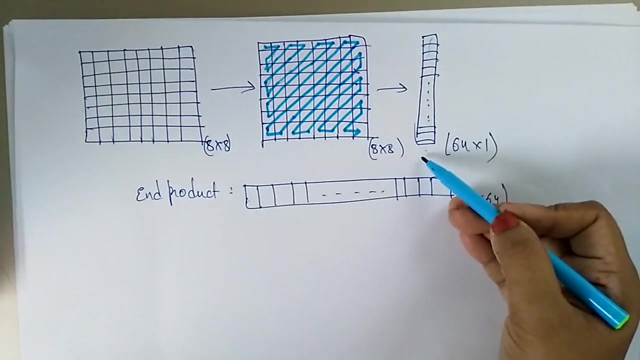 So like this, you have to apply, So see here, This is a zigzag. Let's take: this is a pixels, So apply the zigzag technique, So whatever the applying zigzag technique, So that numbers will be written like this: It is a one dimensional. You have to write that in a everything The letters.